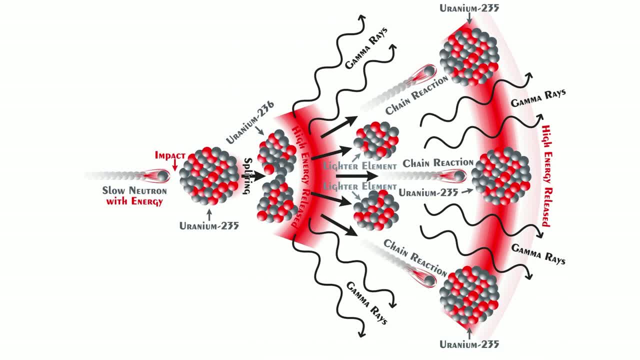 of a large atom like uranium-235 into smaller elements. A neutron strikes uranium-235,, which then becomes a very unstable uranium-236,, which quickly splits into lighter elements and gives off additional neutrons, gamma rays and energy. These new neutrons then strike. 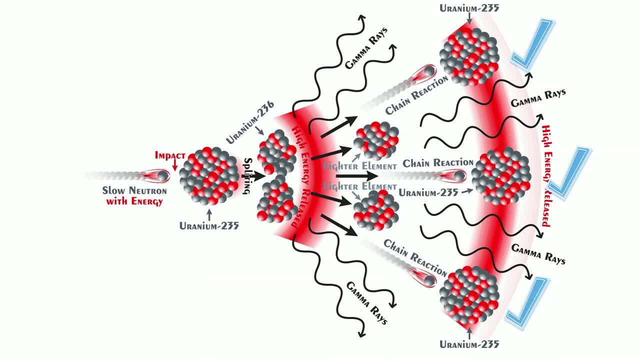 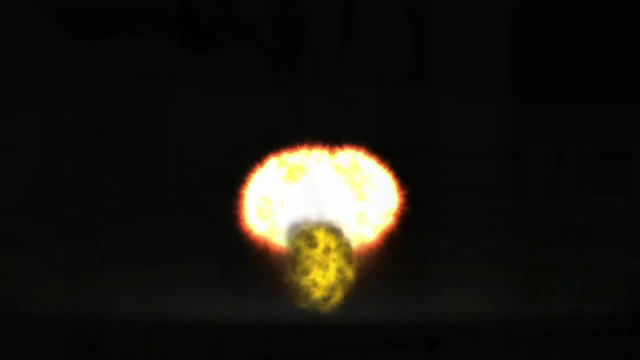 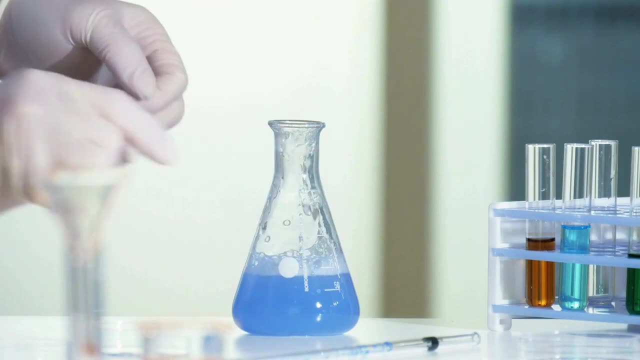 other uranium-235 atoms which repeat this process and this can set off a chain reaction. The energy given off is much greater than a chemical reaction, which makes it a very dense source of energy, but less than nuclear fusion. The products of nuclear fission, like 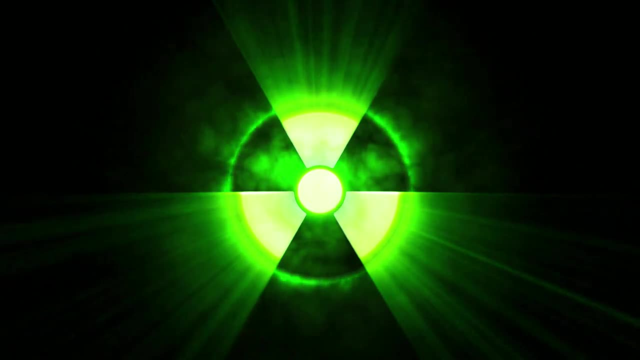 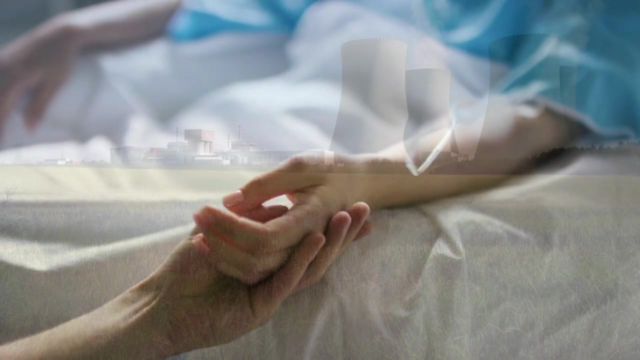 iodine-131,, cesium-137, and strontium-90, are created in this process and can be radioactive for thousands of years. Exposures to each of these elements can cause sickness, cancer and even death. The heat from nuclear fission can be used to heat steam, which in turn turns a turbine. 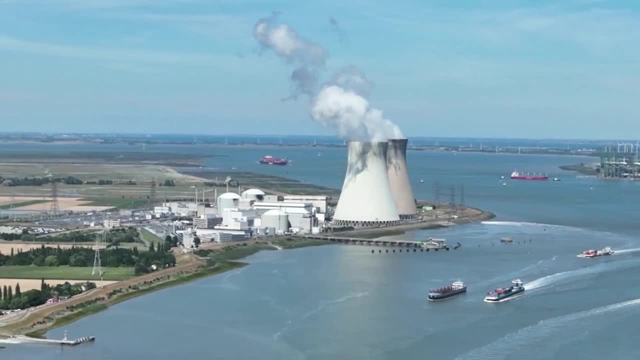 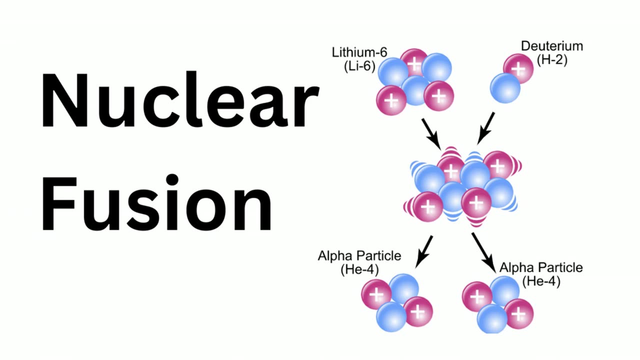 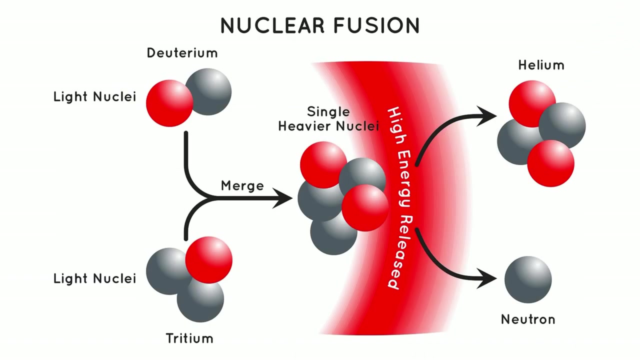 to produce electricity. Currently, there are 439 nuclear reactors in operation in 30 countries around the world. On the other hand, nuclear fusion is the combining or fusing of two or more lighter elements into a larger one. For example, two isotopes of hydrogen, deuterium and tritium, will. 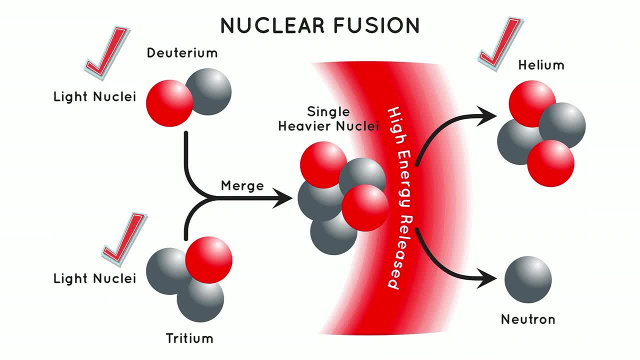 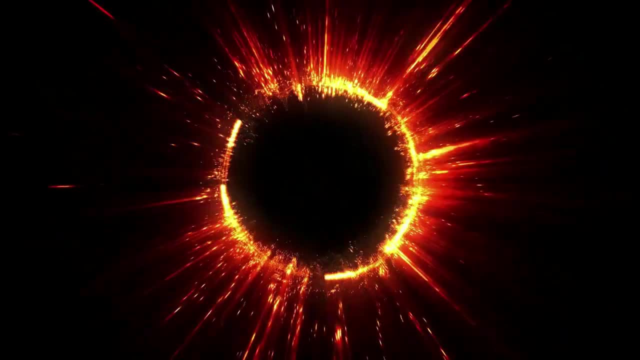 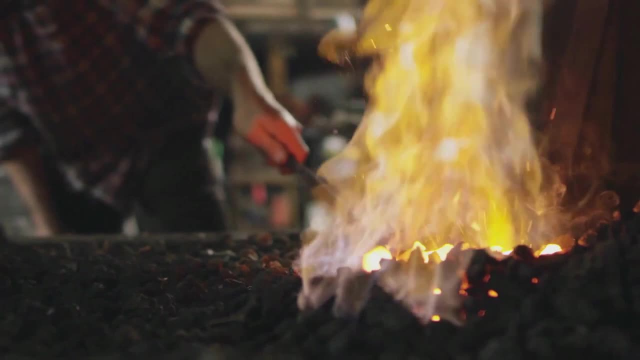 fuse and produce helium and give off one neutron plus lots and lots of energy. It takes considerable energy to force nuclei to fuse even those of the lightest elements. It is estimated that on Earth a temperature of 100 million degrees Celsius would be needed. 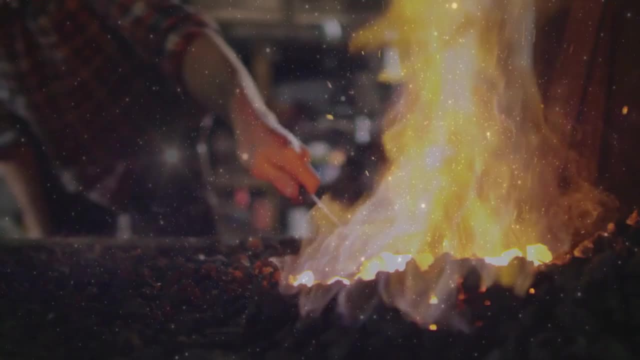 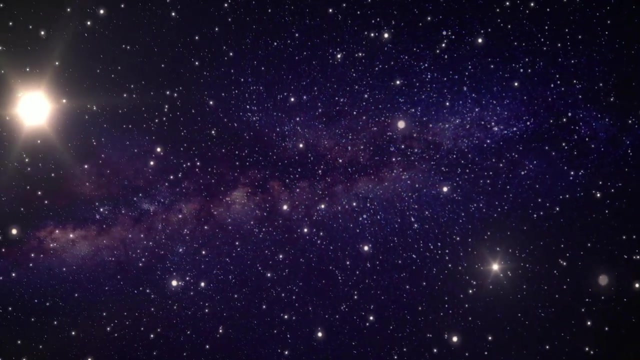 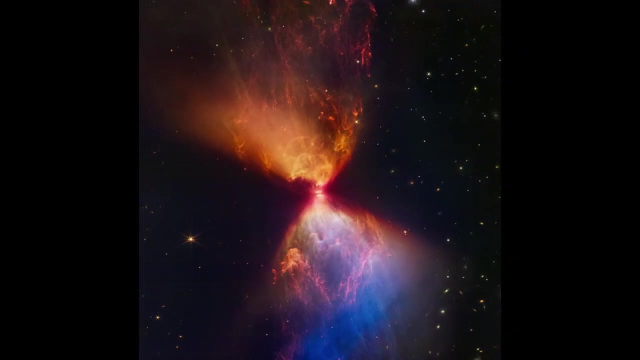 to fuse hydrogen into helium. Nuclear fusion is the energy source of stars, But how does this happen? A protostar is a very young star. The energy released from the collapse of gas into a protostar causes the center of the protostar to become extremely hot When the core is hot enough. 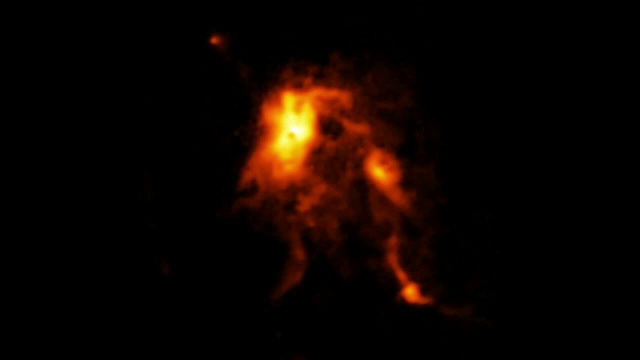 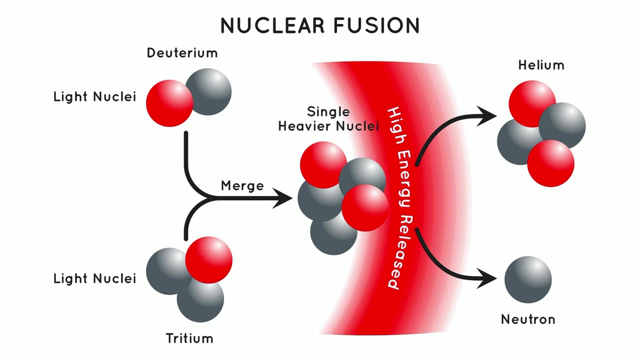 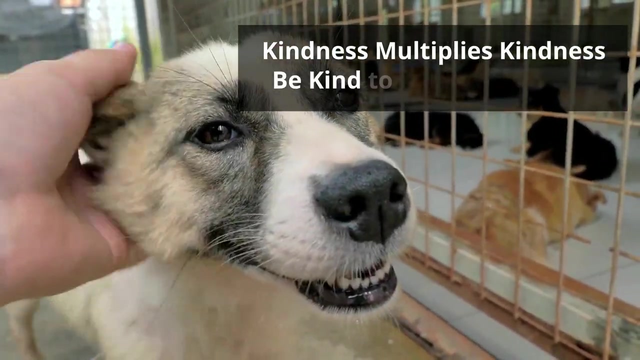 nuclear fusion begins. Nuclear fusion is what created the elements of the stars. Nuclear fusion creates more energy than nuclear fission and does not create the radioactive byproducts. Thanks for watching and remember… Kindness multiplies kindness. Be kind to someone today.